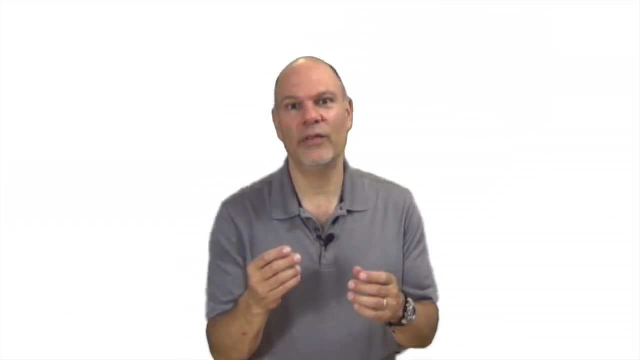 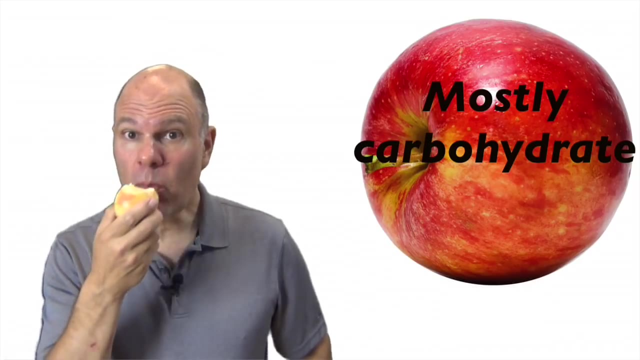 systems. Just think of yourself. a great example of a living system You take in food. Food is a chemical substance made of atoms combined into molecules. That's chemistry. When you digest that food, you take it and you break it down into simpler forms, some of which. 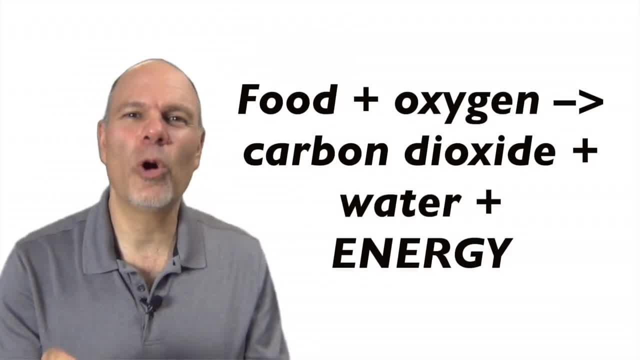 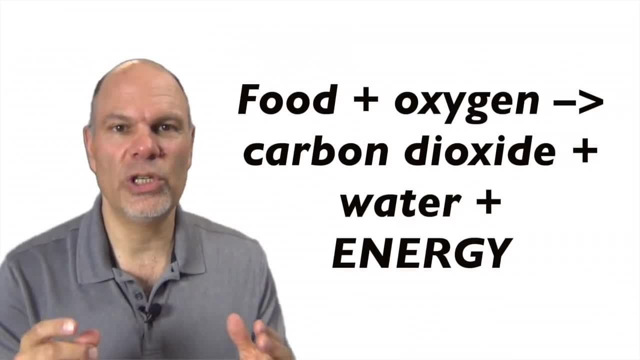 gets made into you. That's chemistry. You'll take other parts of that food, you'll combine it with oxygen and you'll make it into molecules that your cells can use to do the work of life. That's chemistry too. It's all chemistry. We're going to start our study of chemistry. 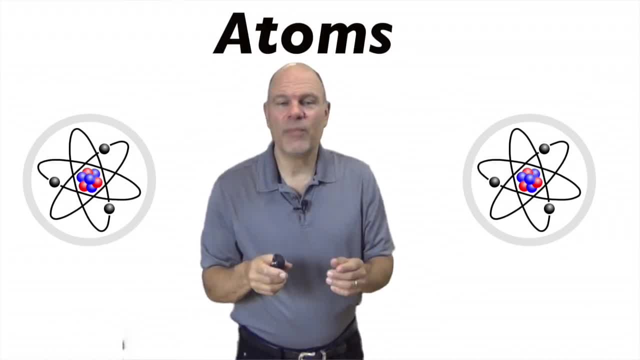 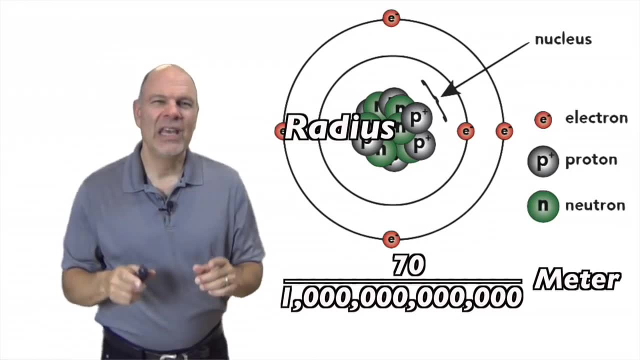 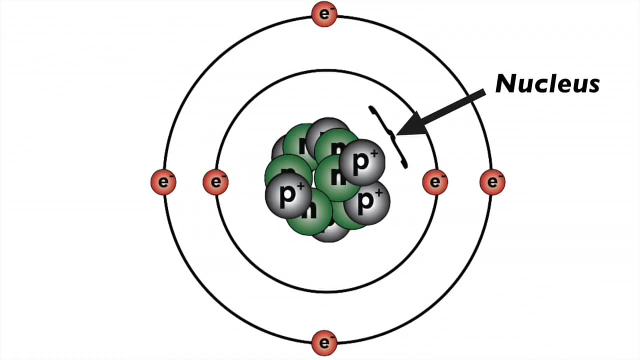 by looking at atoms. Atoms are the building blocks of matter. They are unimaginable. The radius of a carbon atom, one of the most important atoms in living things, is 70 trillionths of a meter. Almost all the mass of an atom is found in a dense core called the nucleus. 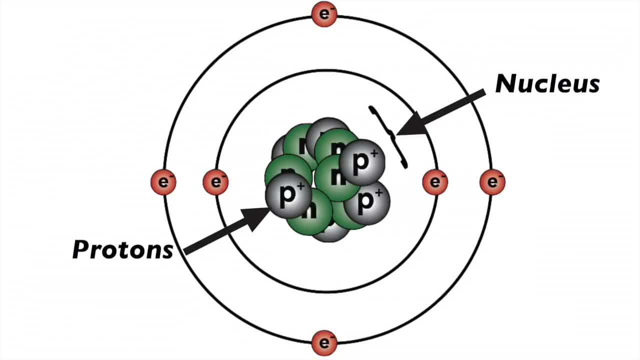 The nucleus is made up of positively charged particles called protons and other particles called neutrons that have no charge at all. Orbiting outside of the nucleus way in the distance are negatively charged particles called electrons, which have very little mass. I've just used the term charge. 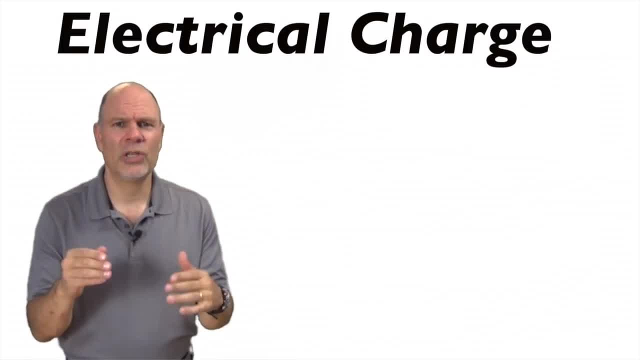 What does that mean? What do you need to know? You don't need to know very much. Charge is a fundamental property of certain particles. Particles like protons have a charge. Particles like electrons have a charge too, and neutrons don't. What you need to know as a biology? 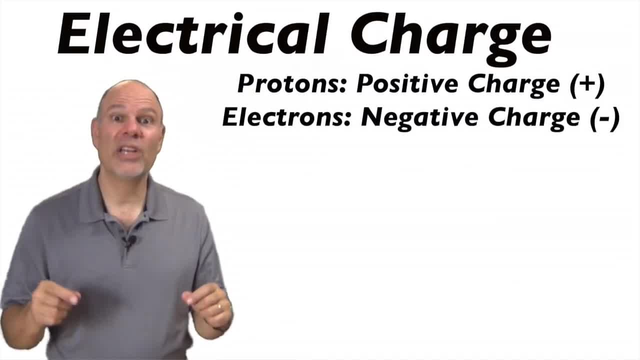 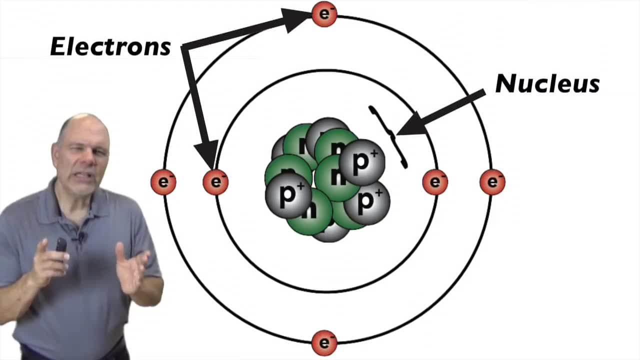 student is that protons have a positive charge, electrons have a negative charge, that, like charges, repel and that, unlike charges, opposite charges attract. In this representation of a particle, electrons are like a miniature solar system. The nucleus is about where the 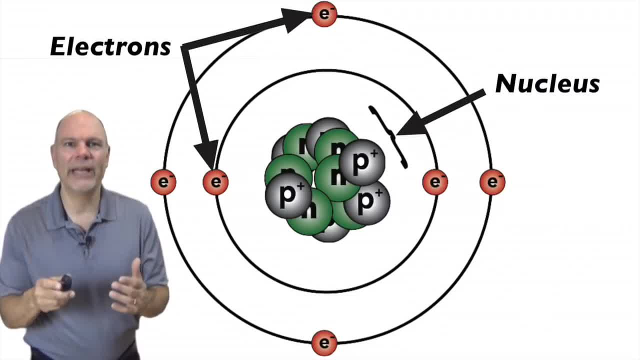 sun would be, and the electrons are shown kind of like planets orbiting outside. The reality of atoms is much more complex and when you take chemistry you'll learn a much better model, but you don't need that for now. The region where electrons are found has three names. They're called orbitals, You can remember. 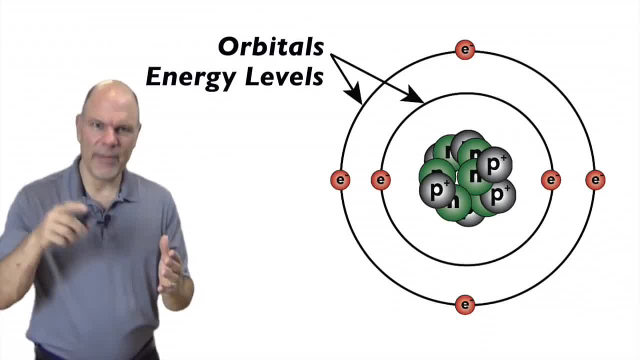 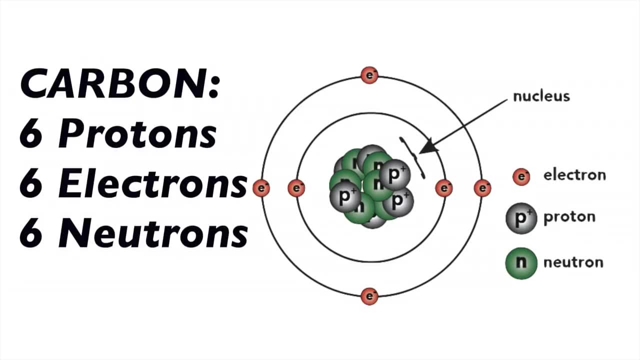 the word orbit. They're called energy levels, and we'll see that's because the amount of energy is corresponding to where they are, and they're also simply called shells In this example. this is a very simple principle: The number of protons and the number of electrons. 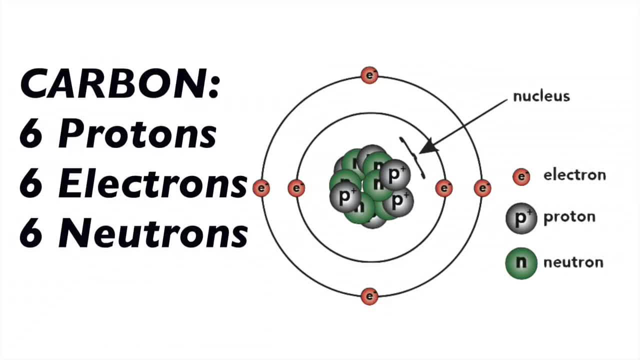 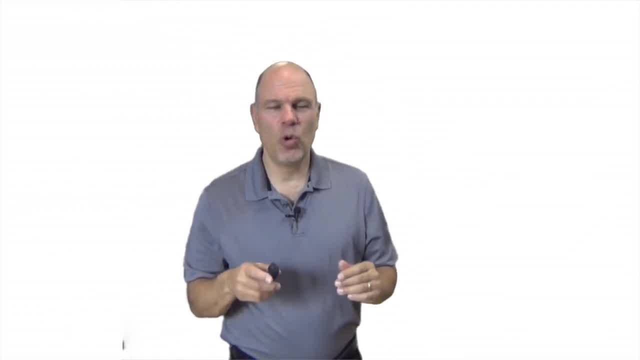 is equal. The number of neutrons is usually about the same as the number of protons, but it can vary. We'll learn about what it means for an atom to have a charge later on in this course, and we'll also learn about the importance of variations in the number of neutrons. All 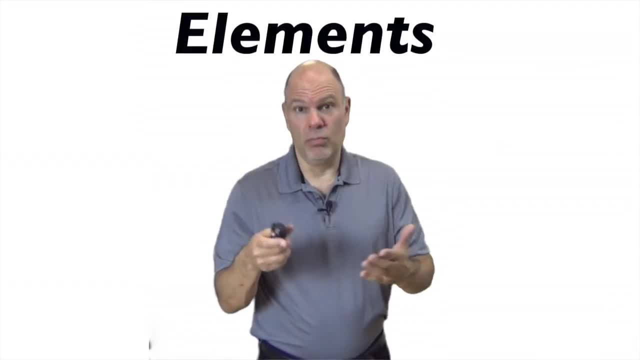 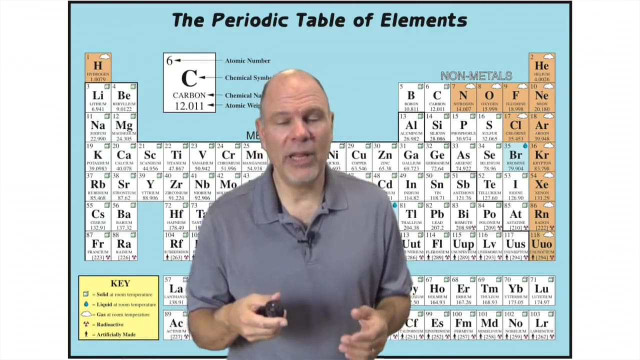 the atoms that have the same number of protons are considered to be the same element. And you've learned about many elements. You've learned about oxygen, You've learned about iron, carbon, hydrogen uranium, so on and so forth. About 90 elements are found naturally on our planet, About a dozen more. 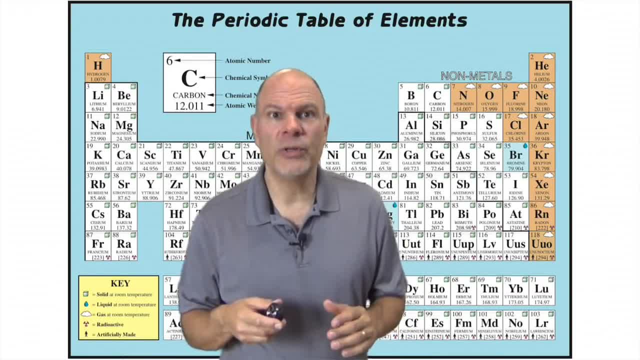 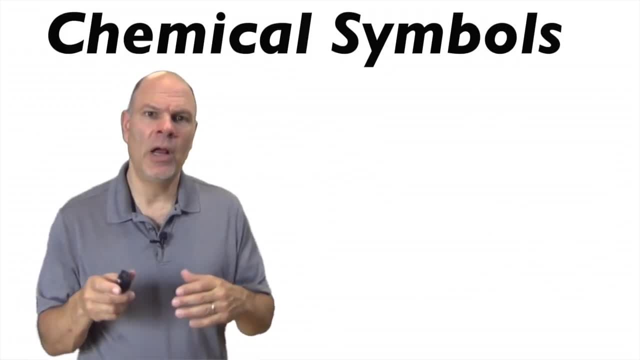 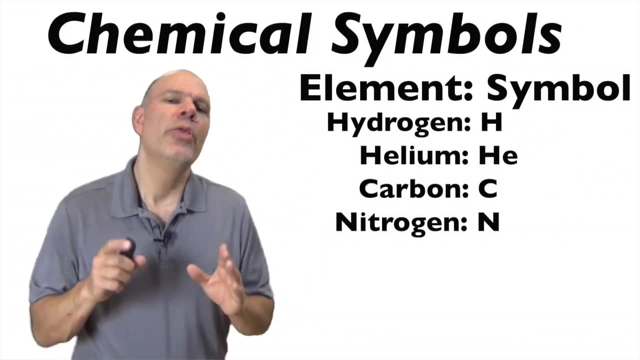 have been cooked up artificially in laboratories around the world. Each element has its own one or two letter chemical symbol, and those are usually pretty easy to remember. Hydrogen symbol is H, helium symbol is HE, carbon symbol is C, nitrogen symbol is N. There are some atoms, however. 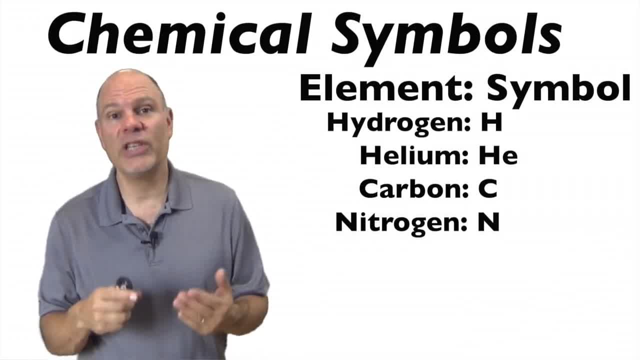 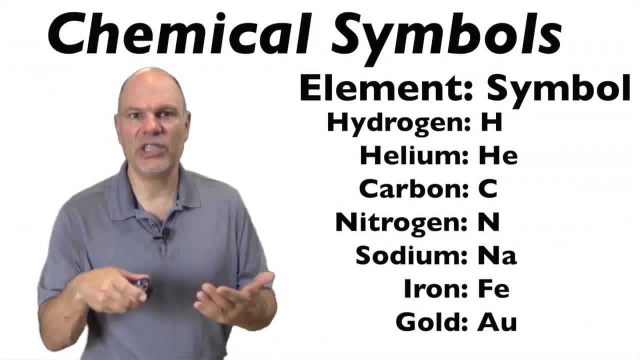 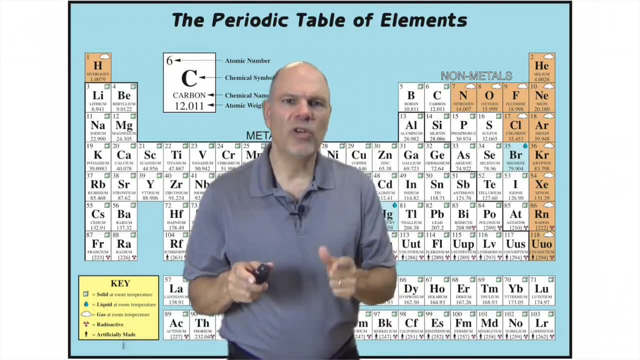 that have chemical symbols that are not derived from English. So, for example, sodium is NA, iron is FE, gold is AU. You'll learn this in the course of your studies of biology and chemistry. The periodic table takes all of the elements and organizes them based on the number. 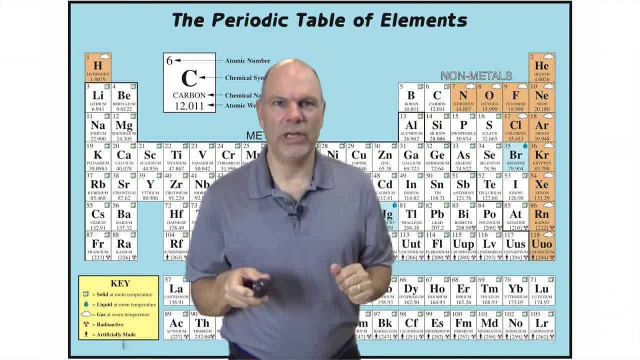 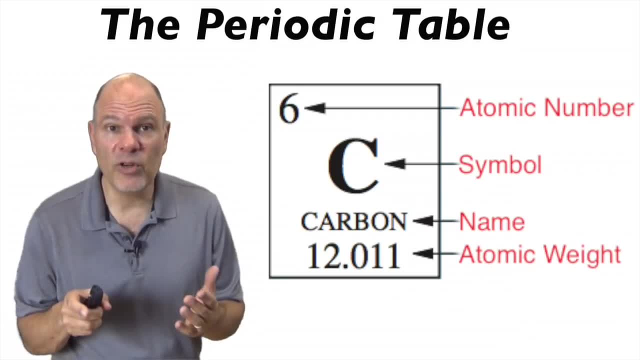 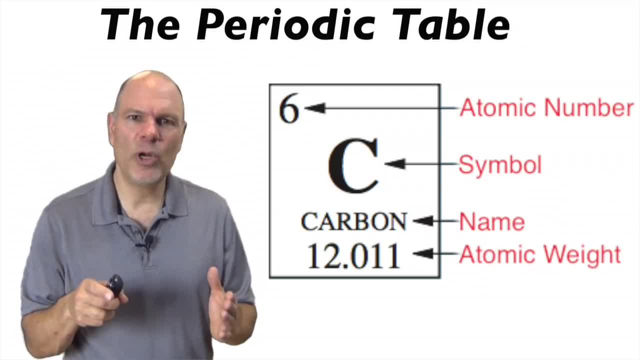 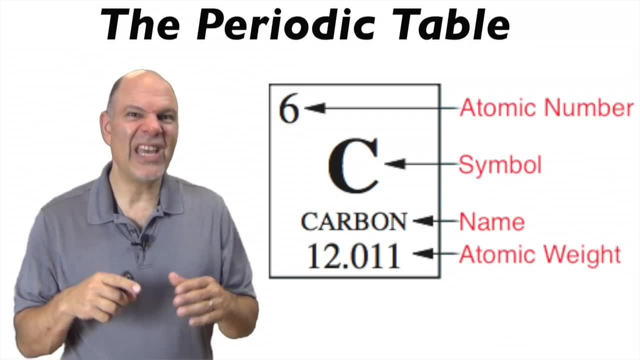 protons, A chemical symbol is the number of protons B, an atomic symbol, which we just discussed- the name of the element and the atomic weight, which is exactly what it sounds like. It's the weight of that atom which you get by adding up the protons, the electrons and the 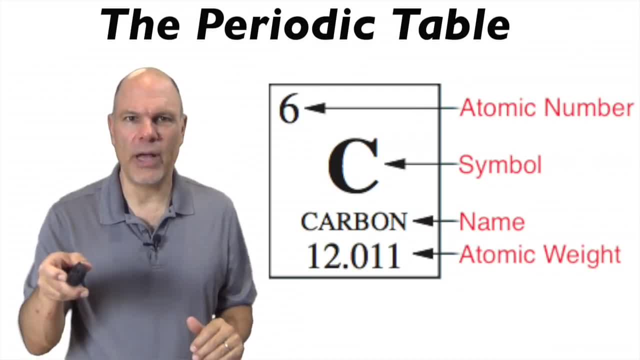 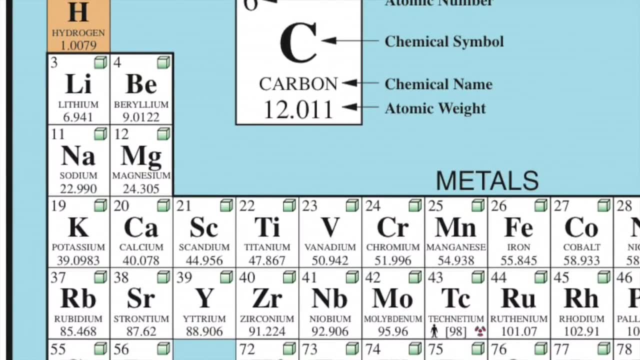 average number of neutrons, which is why it's often not a whole number. The most important thing about the periodic table is how it's organized. Here's what biology students need to know. The number of protons in each element increases from left to right in each. 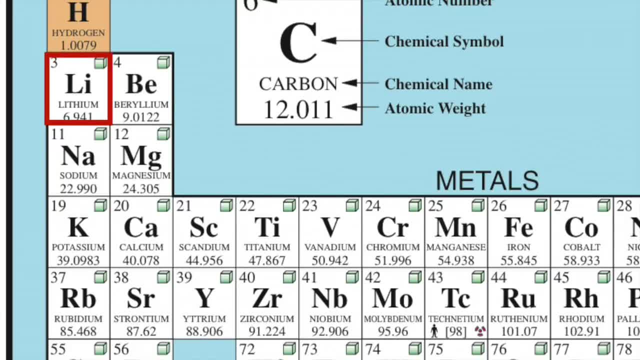 horizontal row. For example, find the second row in the periodic table which begins with it, Li for lithium. Lithium has three protons. The next element, beryllium, with the symbol Be, has four protons. The next one, boron. its chemical symbol is B. you have to jump.